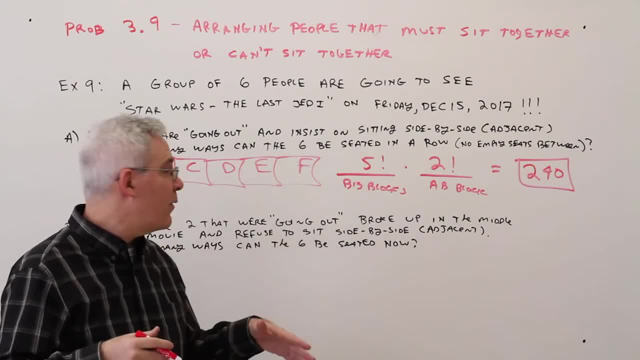 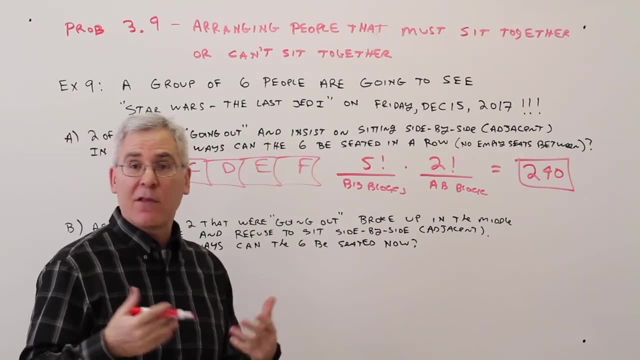 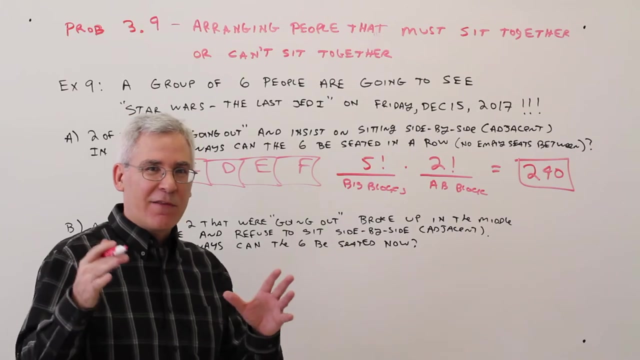 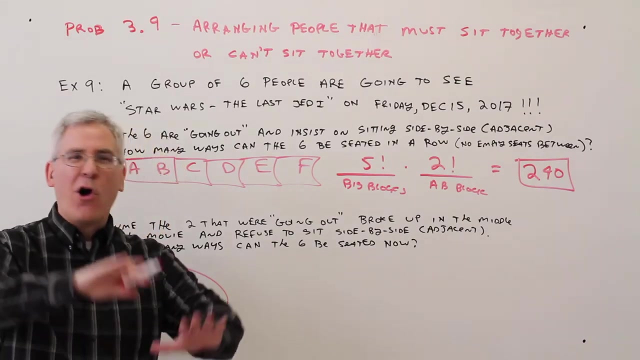 broke up in the middle of the movie. So now they refuse to sit side by side, adjacent. So everybody's got to get up and rearrange themselves. And how many ways can the six be seated now? Okay, so now what I'm going to do is take a slightly different approach. I'm going to draw a set of all possible ways, So the total arrangement. 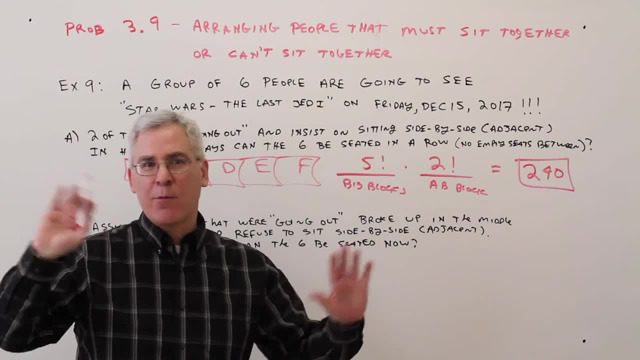 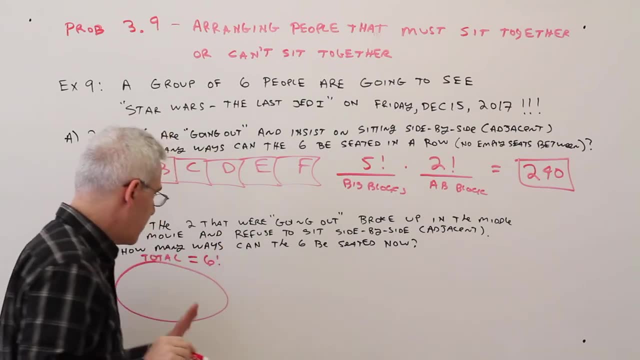 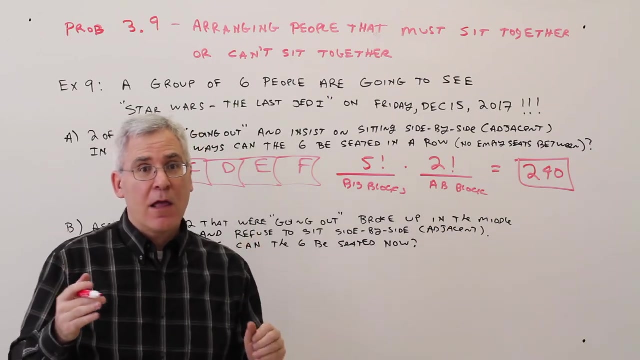 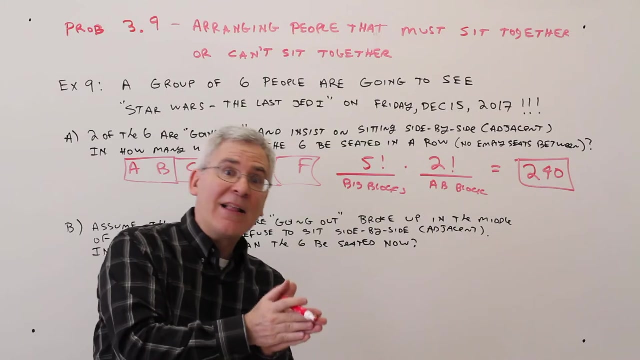 Okay, let's find out what the total arrangements are. Nobody worried about sitting anywhere. Well, there's six people, six factorial, Okay, and then out of those total arrangements, I could break it down into a binary operation. Either A and B are sitting side by side, or A and B are not sitting side by side. It's the same as either it's going to rain or it's not going to rain. 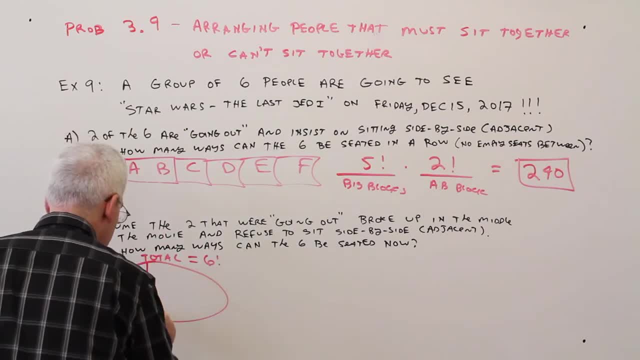 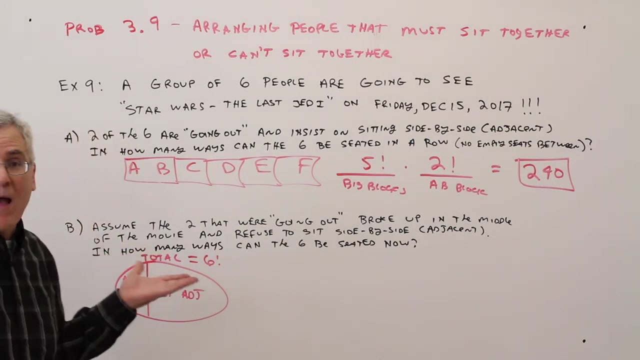 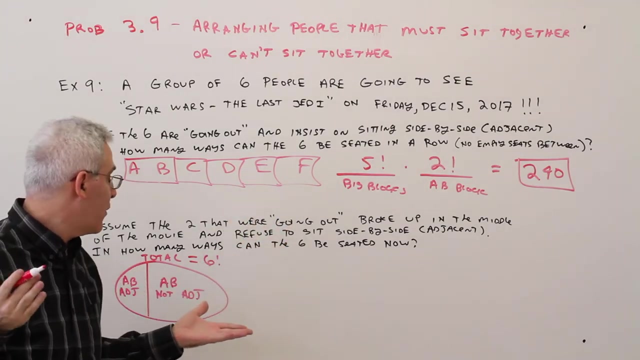 Same concept. So I'll break this set up into two parts. So I'll say A and B adjacent And over here A and B not adjacent. Okay, those are my two possibilities, And I know that they have to sum six factorial. That's the total possible ways. Oh, we just found out the number of ways that A and B are adjacent. 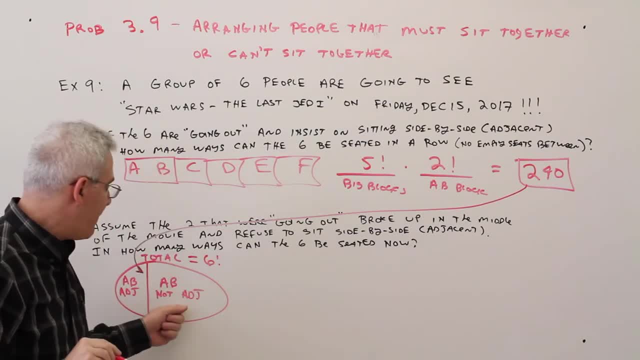 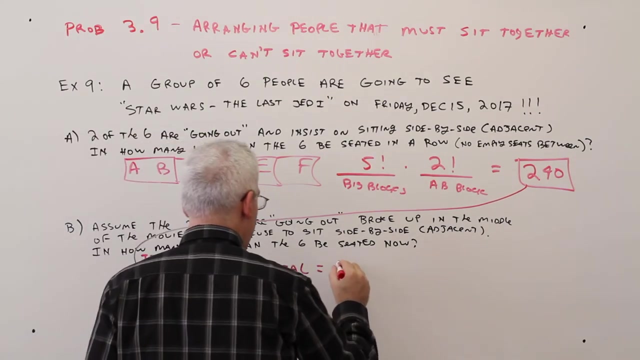 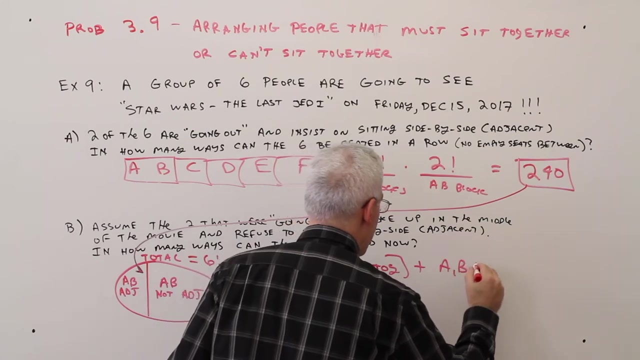 But I want to find out the number of ways that A and B are not adjacent. I can subtract, So I know. I'll just write it the following: I know that the total equals A and B together plus A and B, not together.